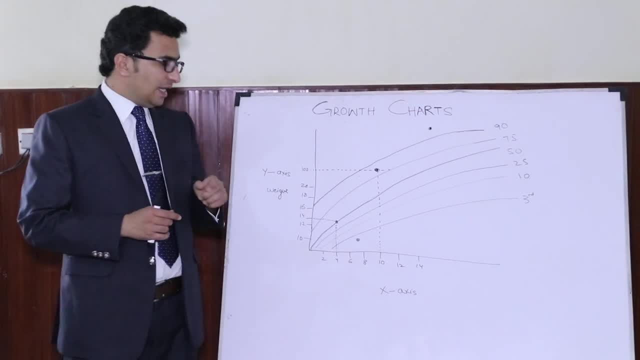 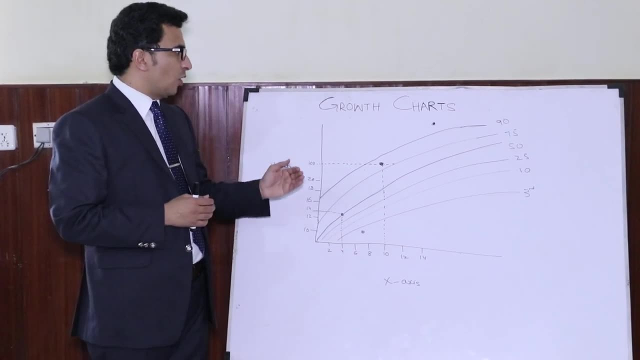 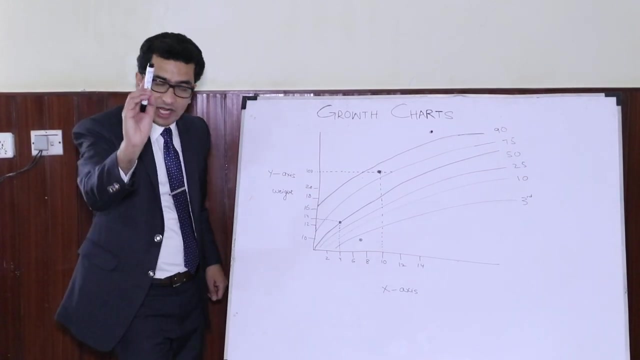 In an examination. if the examiner tells you that you have a 4 year old boy and his weight is 14 kg, please plot it on the growth chart. Then what you need to do? First of all understand that in a growth chart you will have two axis: One is x axis and the other is y axis. 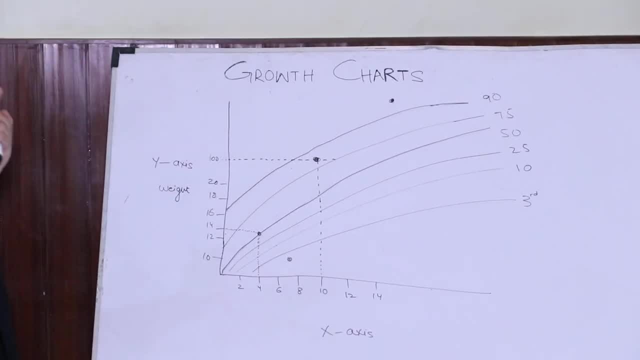 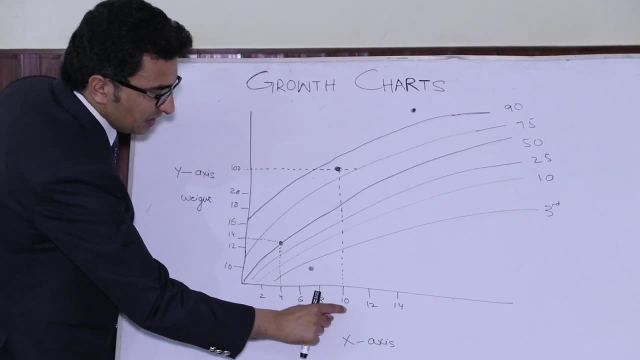 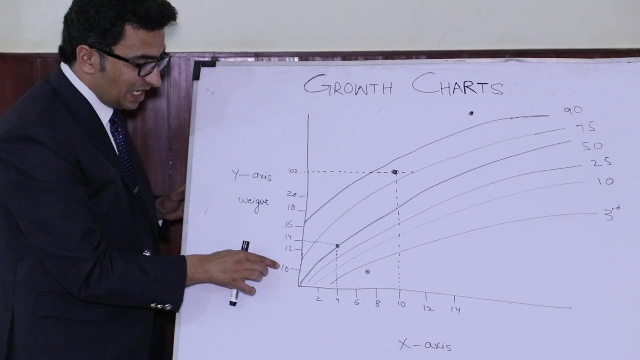 On x axis there will be always different ages already plotted on them, like 2 years, 4 years, 6 years, 8 years, 10 years and so on. On y axis there will always be already plotted weights on it. Let's suppose this is 10 kg. 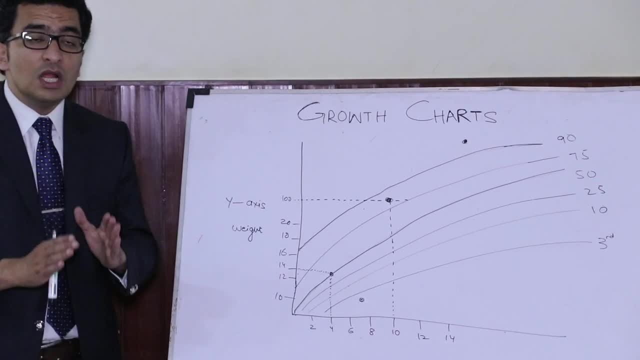 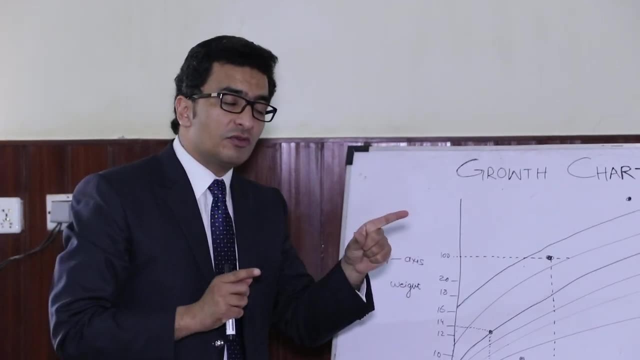 12 kg, 14 kg, 16 kg and so on. Now you will carefully listen to the examiner. You will listen. what is the age of your patient and what is the weight of your patient. Let's suppose he says he is 4 years old and his weight is 14 kg. 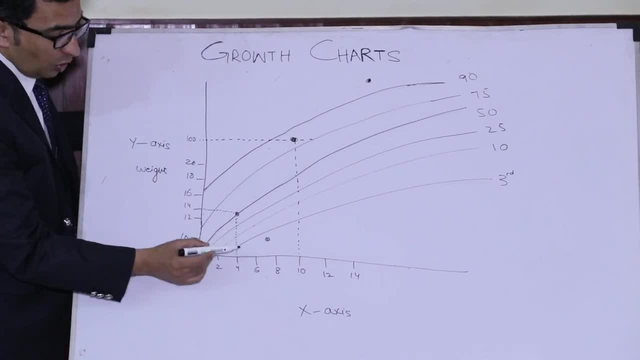 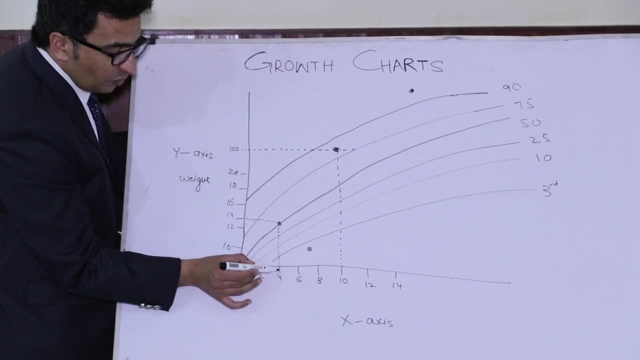 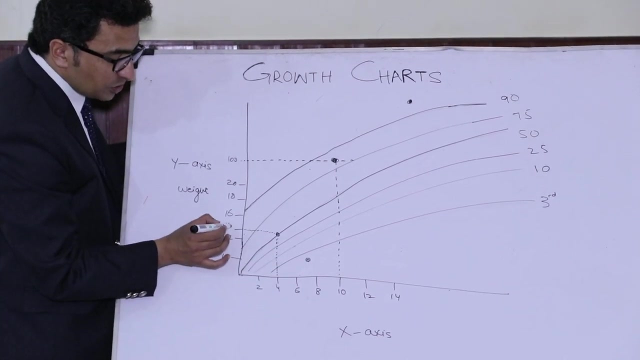 Then what you need to do? You need to put dots, which I have already put over here. You need to put dots from 4 years point. This is 4 years point. You need to put dots Vertically here. Then you need to put some dots from 14 kg point. 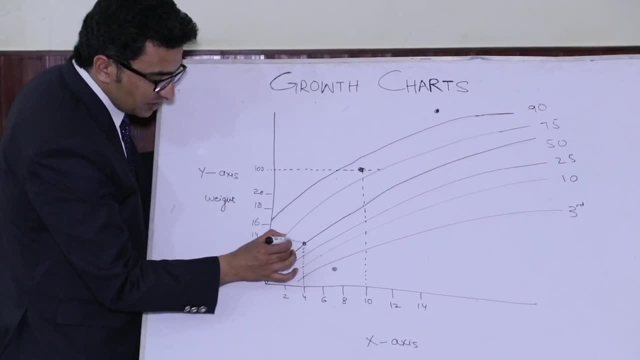 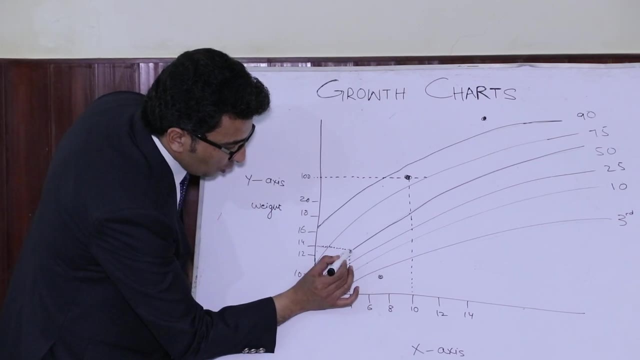 This is 14 kg point. You need to put dot from here. Then you will see where these two dots join. They are joining over here. You will make a big dot over here, Big dot. Then you will see where this dot lies. 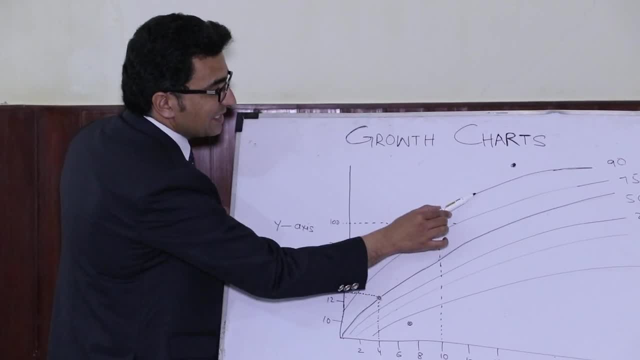 These are different centiles: This is 90th centile, This is 75th centile, This is 50th centile, 25th centile, 25th centile, 10th centile And 3rd centile. 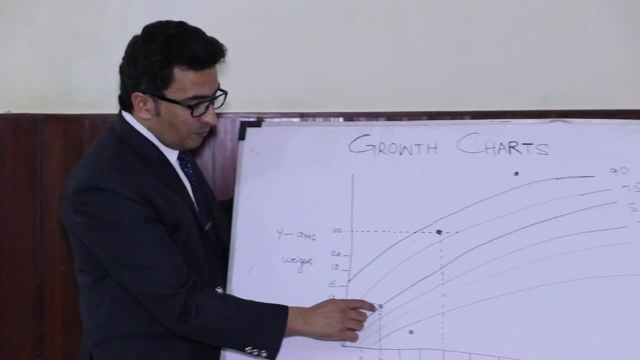 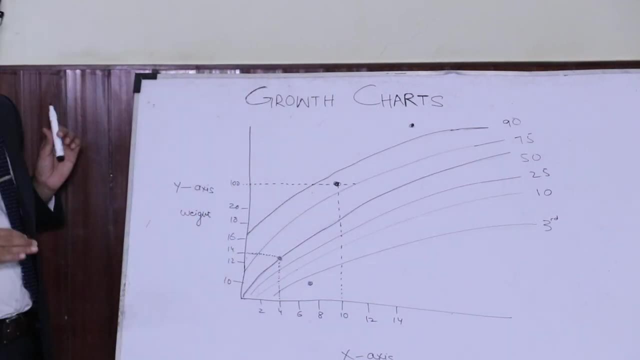 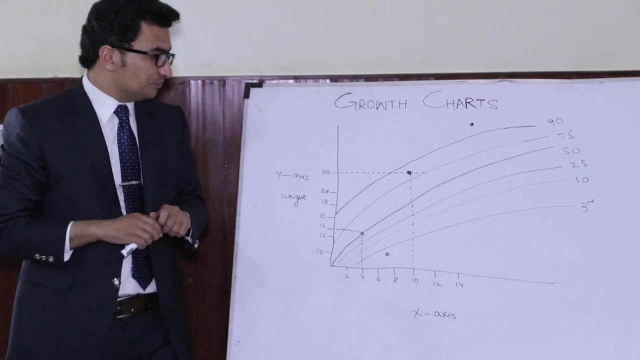 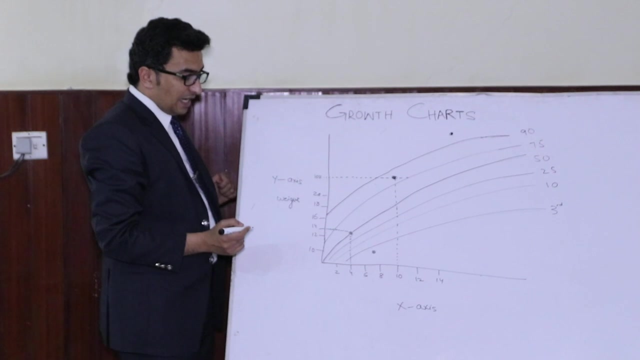 Now you will see where the final dot lies. In this case the final dot lies at 50th centile. So you will tell the examiner that the weight of this 4 years old child lies at 50th centile. Let's suppose if your examiner tells that the boy is 8 years old, 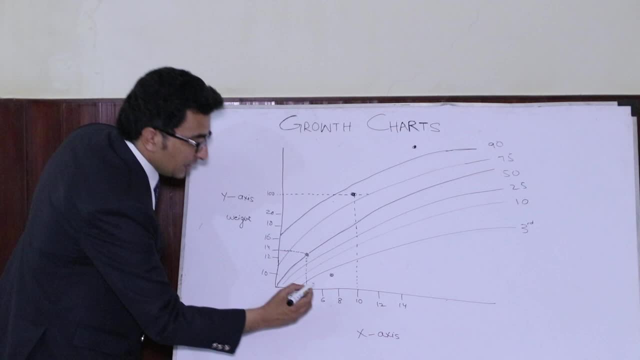 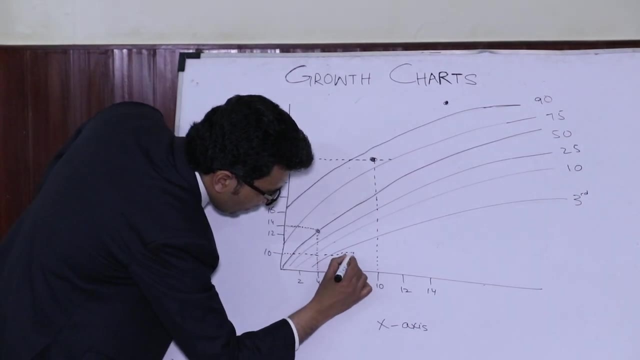 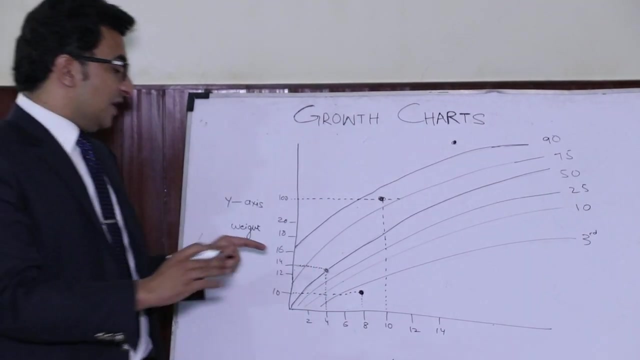 And his weight is 10 kg, Then you need to put dots from 8. And then you need to put dots from 10. And see where the final dot comes. Let's suppose here the final dot comes. Then you will see where the final dot lies. 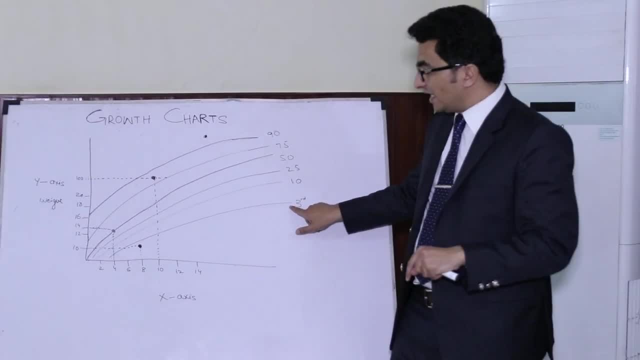 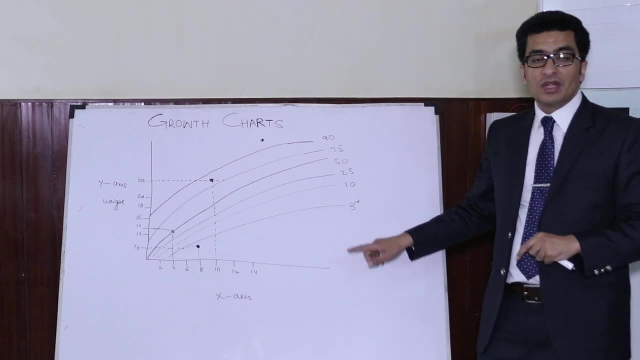 At which centile? This is the 3rd centile, This is the lower most centile. Here is the final dot. You will say that the height of this child lies below 3rd centile. Now let's suppose you have an obese child. 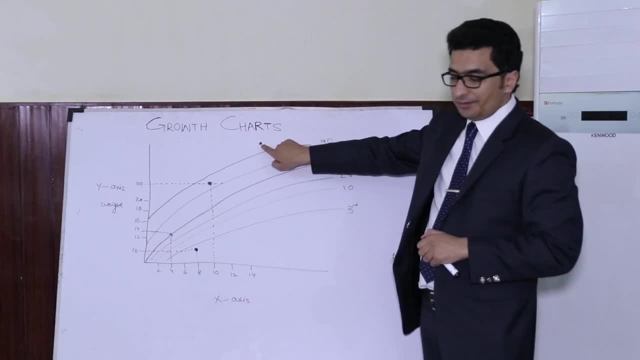 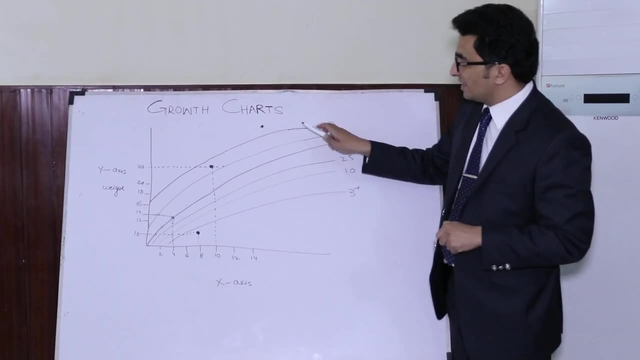 Whose weight lies over here At this point, Then you will say that the weight of this obese child lies above 90th centile. This is the 90th centile. This is the final dot which you have made after putting dots from here and after putting dots from here. 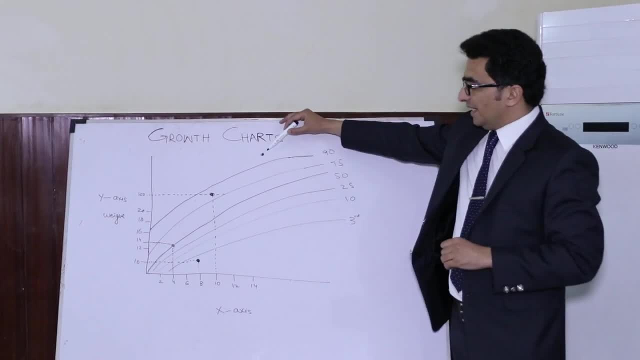 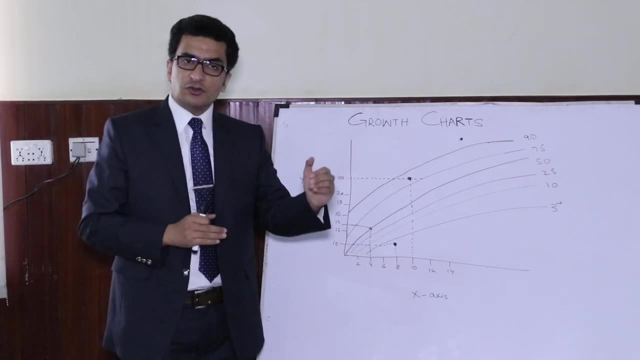 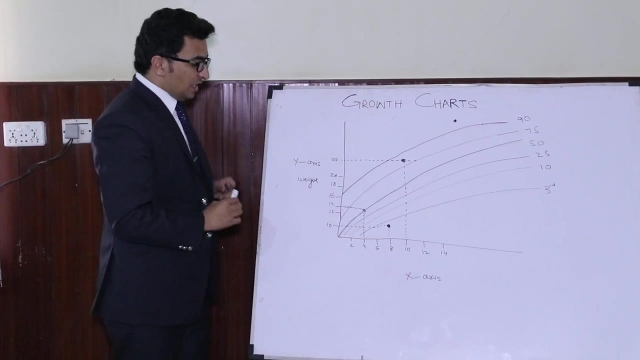 So here you will say that the weight of this child lies above 90th centile. Now if your examiner asks you, Ask you to plot height of the patient, Then the similar growth charts for height will be taken, In which the age will be already on x axis.